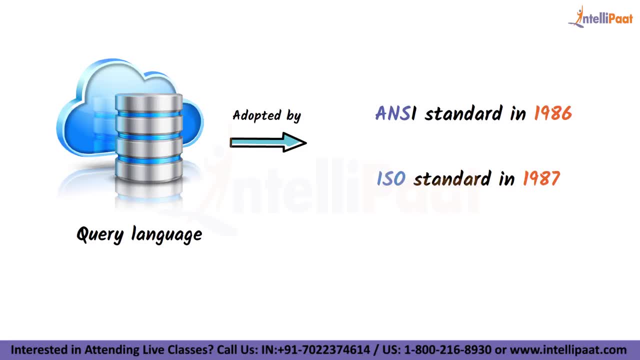 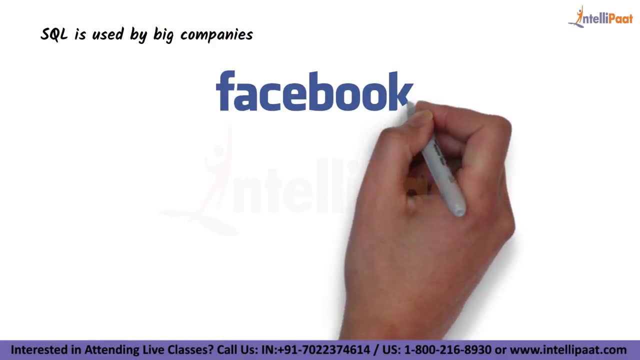 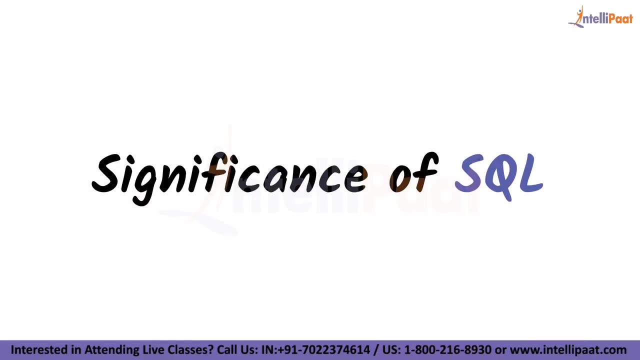 It is the most important query language to learn if you want to work in the field of data science. SQL is used by big companies like Facebook, Instagram and LinkedIn to store data in the backend. So now let's see what is the significance of SQL. A computer programming language, is. 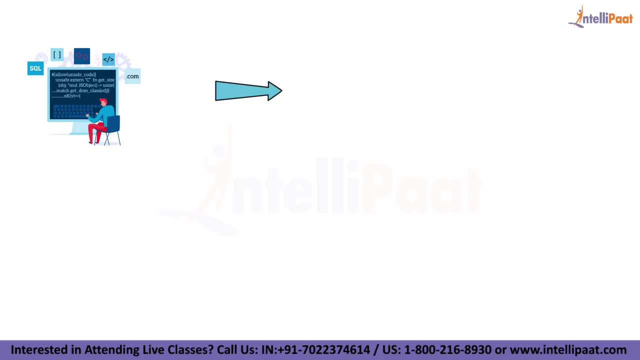 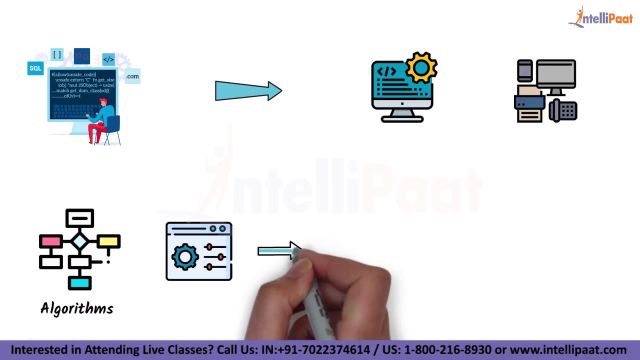 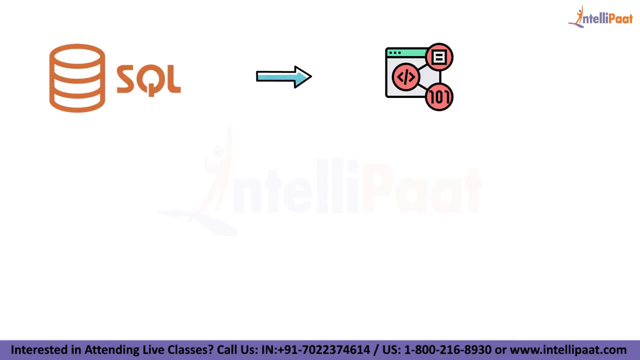 a set of explicit instructions for accomplishing specific operations on computers or equipment. We can use precise algorithms to control the behavior and output of a computer using a programming language. SQL is one such programming language used by the computer. This helps computers and machines to process vast amounts of complicated data more efficiently and effectively. That 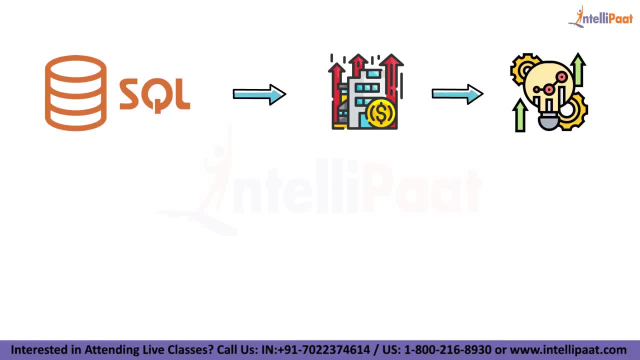 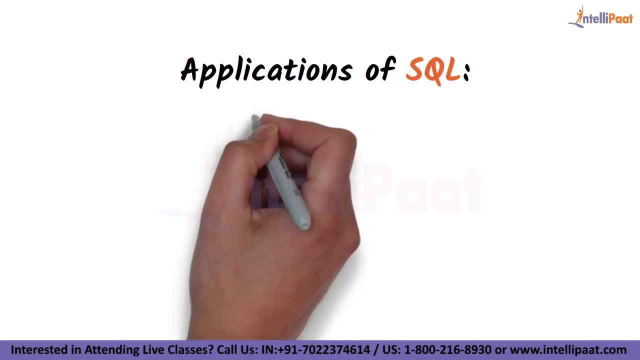 is why SQL is beneficial to business, particularly in the development of system database management services. So let's see what are the different applications of SQL. As previously said, SQL is one of the most extensively used database query languages. SQL is one of the most extensively used database. 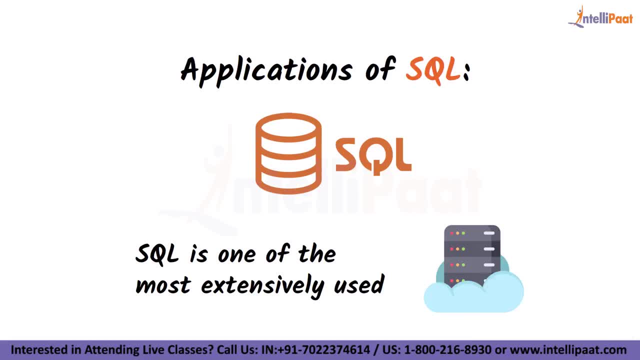 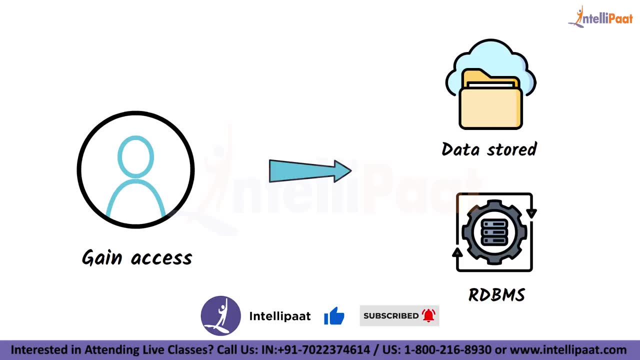 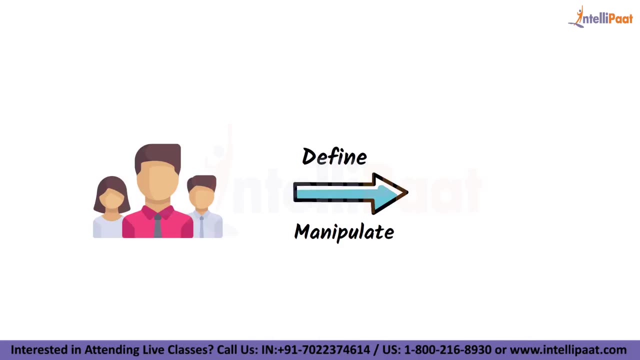 query languages. SQL is one of the most extensively used database query languages. SQL is one of the some of the applications are: the users can gain access to data stored in relational database management systems using SQL. users can use SQL to describe the data. SQL also allows users to define and manipulate the data in a database. it 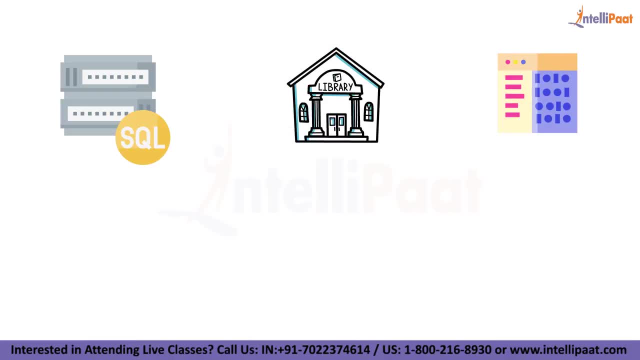 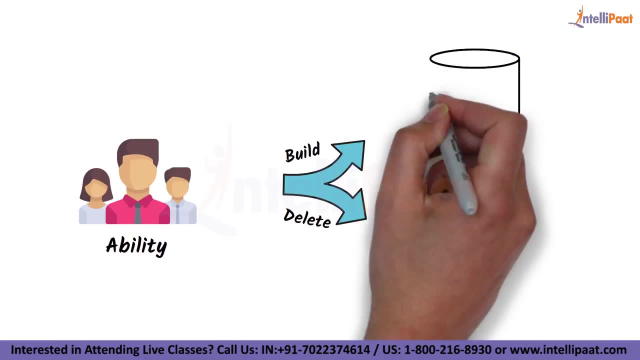 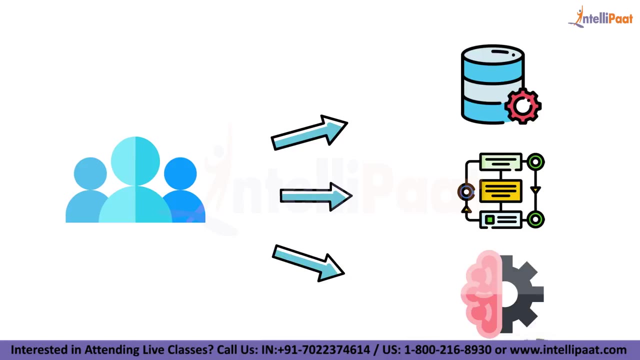 allows SQL modules, libraries and pre compilers to be embedded within other languages. the users can have the ability to build and delete cross database and tables. it also allows users to build database views, stored procedures and functions. permissions for tables, methods and views can be set by the users with 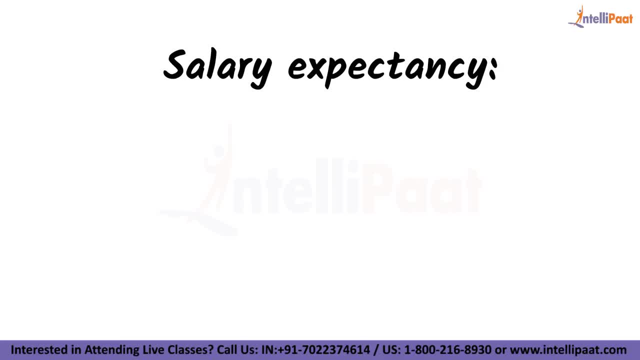 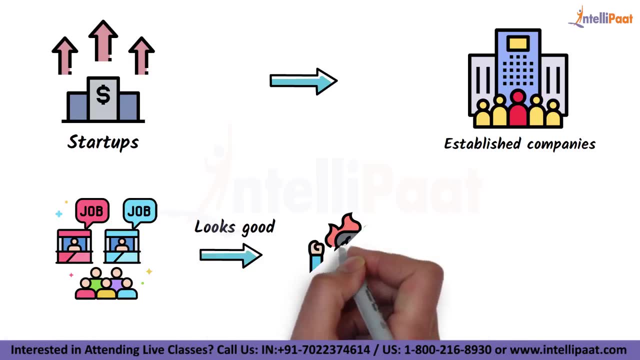 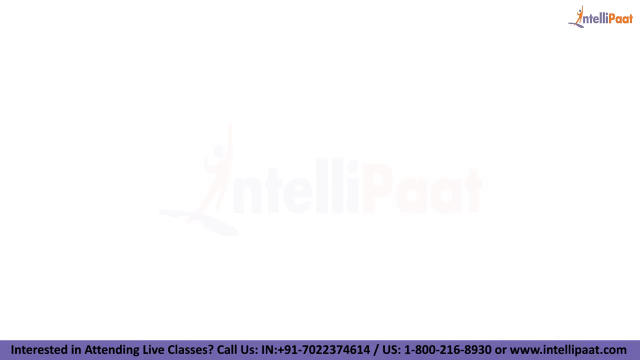 SQL. so let's see what are the salary expectancy of SQL enthusiasts, from startups to established companies. the job market looks good for SQL enthusiasts and it is expected to grow exponentially in the coming years�j� маг program Customers or developers have good opportunities in all the geographies. 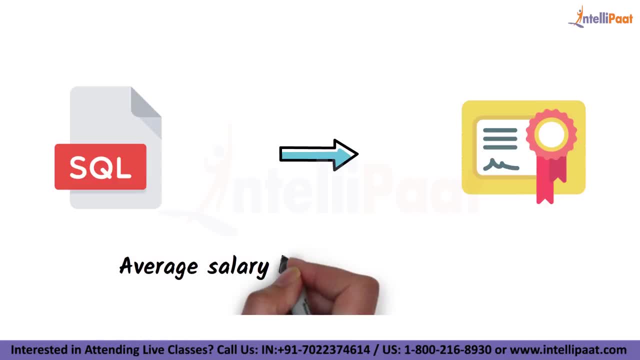 Also, after obtaining a certification in SQL, the average salary hike expected is around 40-50%. So that's all about SQL. Happy Learning.